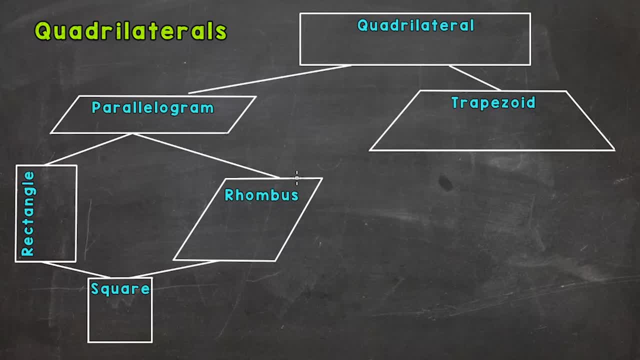 or I added one with all the notes typed out. So use how you see fit and go from there. So I'm going to start up top with quadrilateral. So a quadrilateral is a four-sided square And has to have four angles. 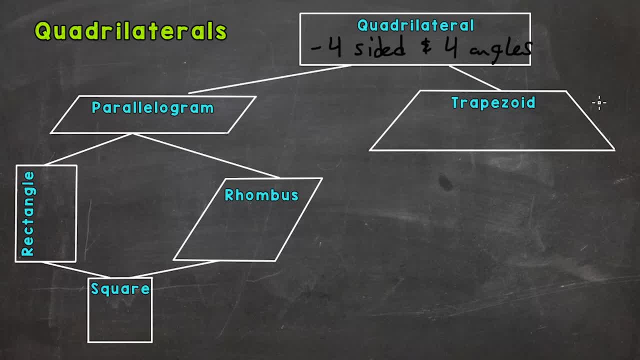 Polygon, So four sides, four angles. Anything that meets that criteria is a quadrilateral. And when I say polygon, that means a flat, two-dimensional shape with no rounded edges and it's closed, No openings. And a quadrilateral is a specific type of polygon. 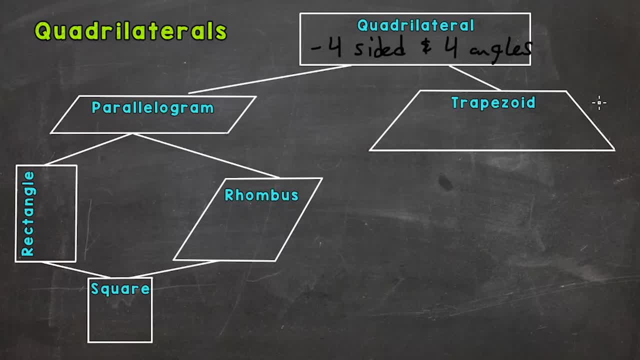 and then now we're getting into more specific types of quadrilaterals. So anything with four sides, four angles, One side, 2 sides, one angle, two sides, quadrilateral sides, four angles, quadrilateral. So as we work our way down, we're going to veer off to the right. 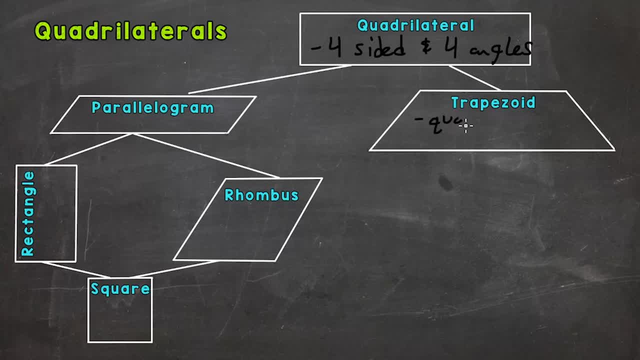 here to trapezoid. So a trapezoid is a quadrilateral, but it also has to have one pair of parallel sides. So in the trapezoid that I'm writing in, the top and the bottom are parallel. 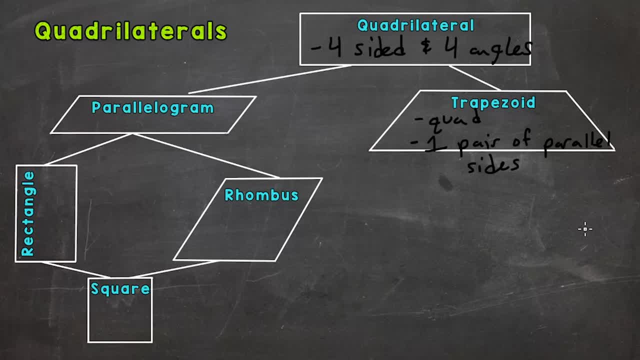 the left and the right or not. So we have a trapezoid, exactly one pair of parallel sides. Now, if we go to the left, we have a parallelogram which is a quadrilateral. but a parallelogram has to have two pairs of parallel sides. 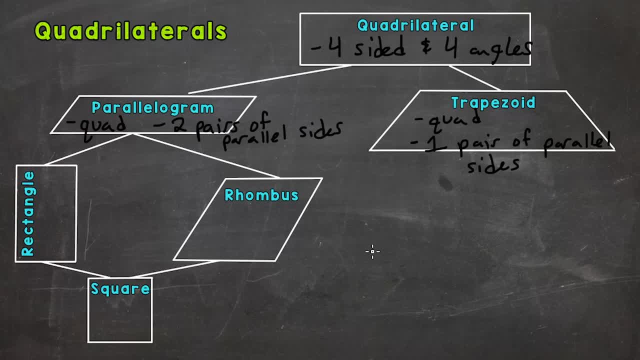 Okay, so we're getting a little more specific as we work our way down. Now let's go to rhombus here. So rhombus is a quadrilateral, It is a parallelogram, so it has to have two pairs of parallel sides. but we're going to give. 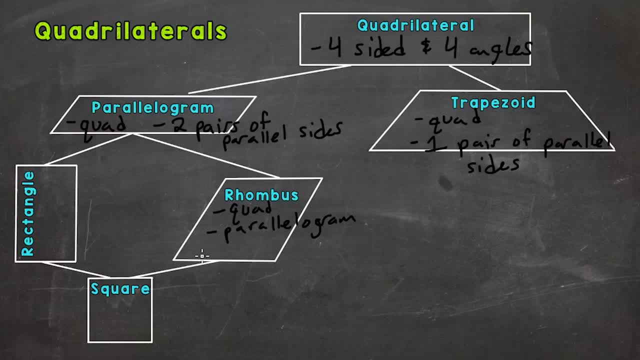 it one more specific characteristic: A rhombus has four congruent sides, and congruent means equal. All sides have to be equal. So if a shape is a quadrilateral, it has two pairs of parallel sides and four congruent sides. all the sides are the same. the best name for that shape is rhombus. 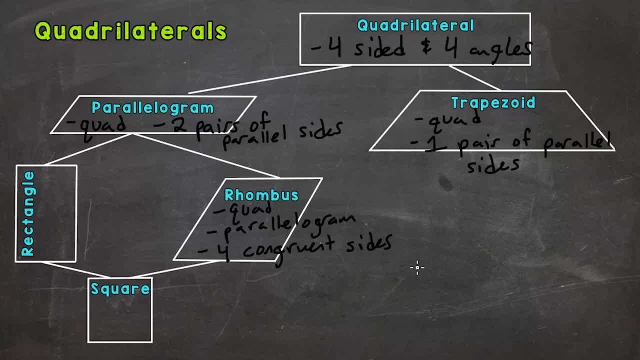 The best name for that quadrilateral is rhombus. You could also call it a quadrilateral. It is a quadrilateral, but the best name is rhombus. Now let's take a look at rectangle. A rectangle is a quadrilateral. It has four sides, four angles. It is a parallelogram. It has two pairs of parallel. 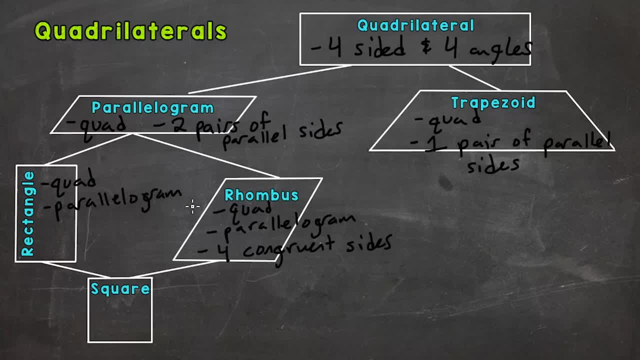 sides. but what makes it more specific than a parallelogram and a quadrilateral? it has to have four right angles, So four 90 degree angles. Now, the most specific quadrilateral is a quadrilateral. It has four sides, four angles. 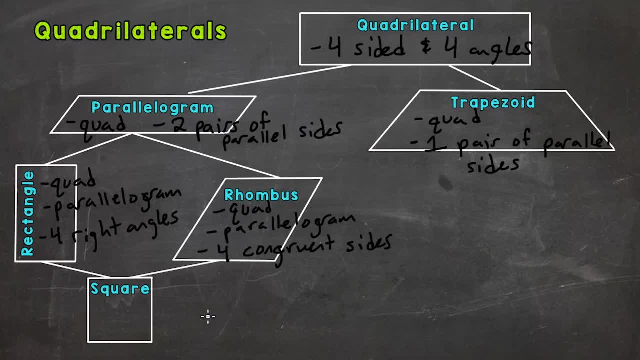 The most specific quadrilateral of all is the square. So a square basically combines everything on the left side of your screen: the parallelogram, the rectangle and the rhombus to make the most specific quadrilateral, So a square. I'm going to write outside the square here so I have more room. It is a quad, It is a parallelogram. It does have two pairs of parallel sides. 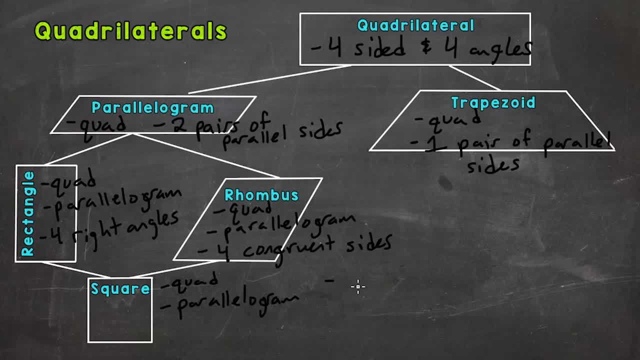 It is a rectangle right, It has to have four right angles And it also has to mix in a characteristic of rhombus: It has four congruent sides. So the best name, if a quadrilateral meets all of those characteristics, would be square. 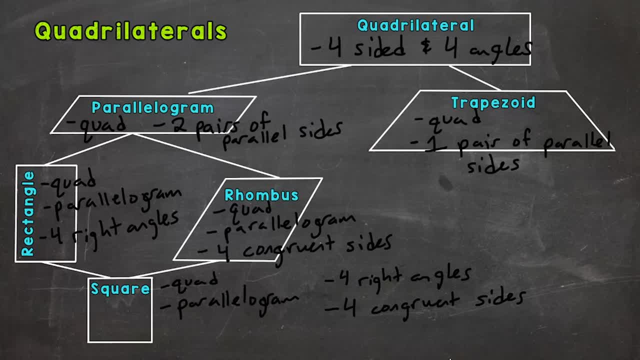 Now, is a square, a quadrilateral? Yes, it has four sides, four angles. Is it a parallelogram? two pairs of parallel sides? Yes, Is it a rectangle? It has those four right angles, plus a quad, plus a parallelogram. Yes, it is a rectangle. 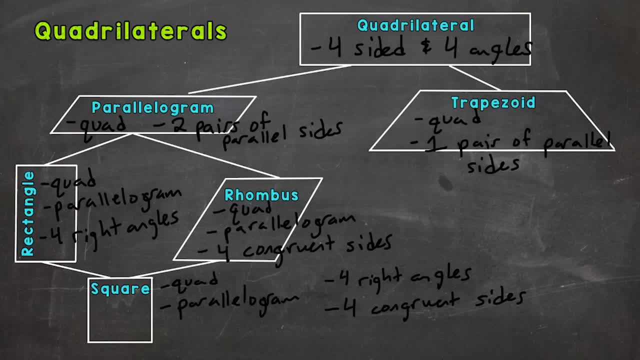 Is it a rhombus quad parallelogram and four congruent sides? Yes, But the best name for it is square. So there are the different types of quadrilaterals. Now, there are some different ones and other ones, but these are the main ones we cover in fifth grade here.